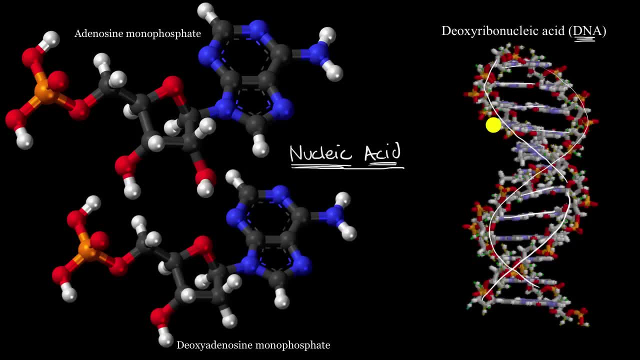 A DNA molecule, let's say in the human genome, a chromosome, for example- is primarily a really long DNA molecule and it can have a long DNA molecule and it can have on the order of 100 million rungs to this ladder. 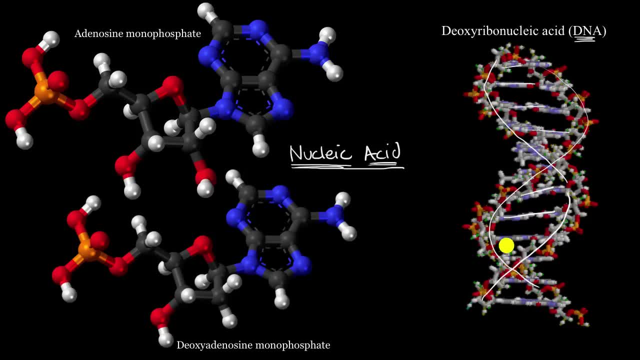 Now another thing to appreciate. like many other macromolecules, DNA or nucleic acids in general, they are polymers, in that they are made up of building block molecules and those building blocks for nucleic acids- and DNA is the most famous nucleic acid- 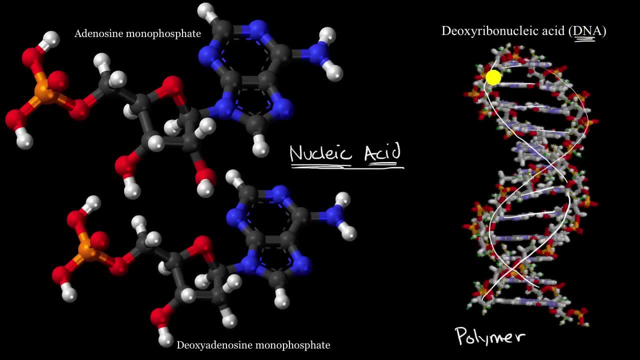 and RNA ribonucleic acid would be a close second, but the building blocks of them are known as nucleotides, And we see some examples of nucleotides right over here. This is deoxyadenosine monophosphate. 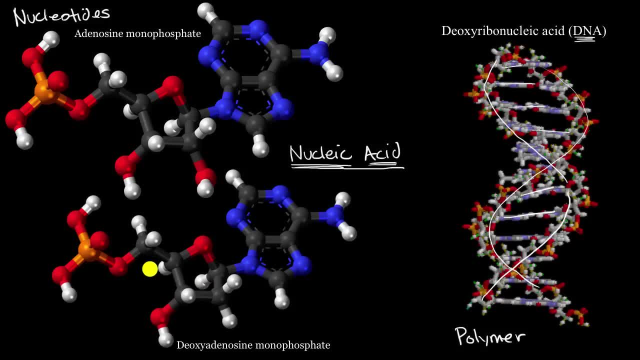 which would be a nucleotide found in DNA. You can see the various parts of it. You have a phosphate group right over here. You have a five carbon sugar, which in this case is ribose, and then you have what is known as a nitrogenous base. 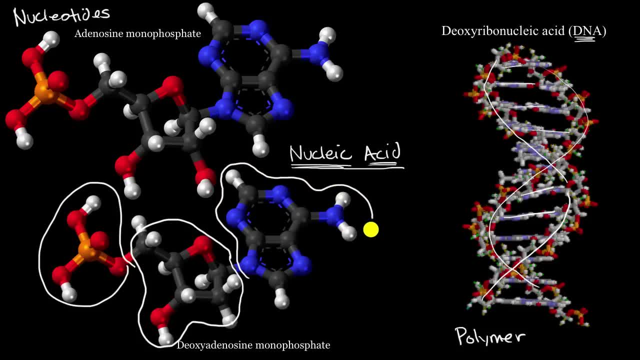 and why is it called nitrogenous? Well, those blue circles represent the nitrogenous base and the red circles represent the nitrogen, and we've seen this before. The grays are carbons and the reds are oxygens and the whites are hydrogens. 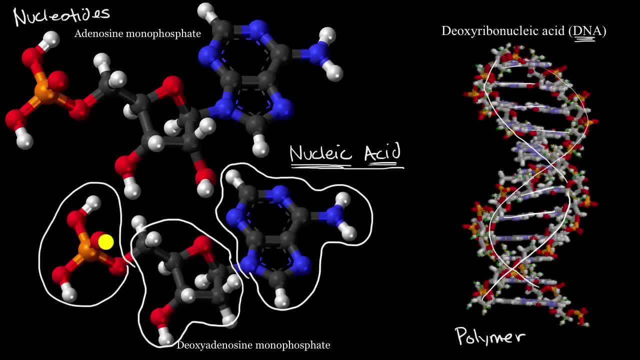 and so this part of the molecule has some basic characteristics, while this phosphate group, at the end this has some acidic characteristics, and what happens is is they get stacked onto each other, where the ribose-phosphates alternate to form the backbone of this DNA molecule. 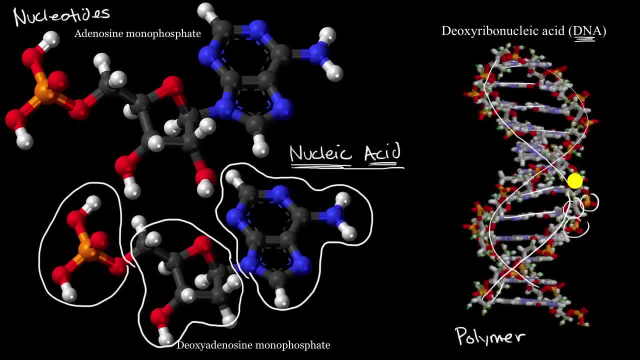 You can see it right over here, where you have a phosphate and a ribose and a phosphate and a ribose, and then you have the nitrogenous base forming part of the rung of the ladder, and the way that DNA stores information is. 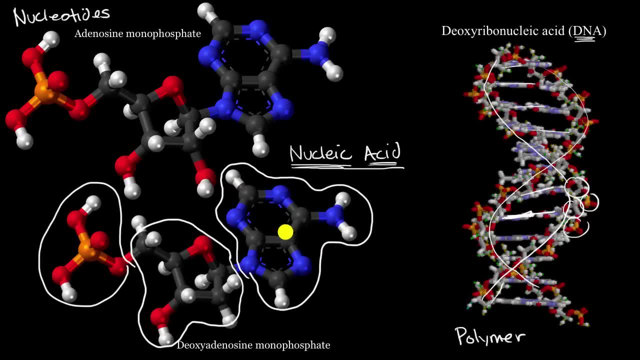 every one of these nitrogenous bases right over here. this is adenine. it has a complementary nitrogenous base on the other to complete that rung of the ladder. so adenine matches with thymine in DNA and we'll see in future videos in RNA. 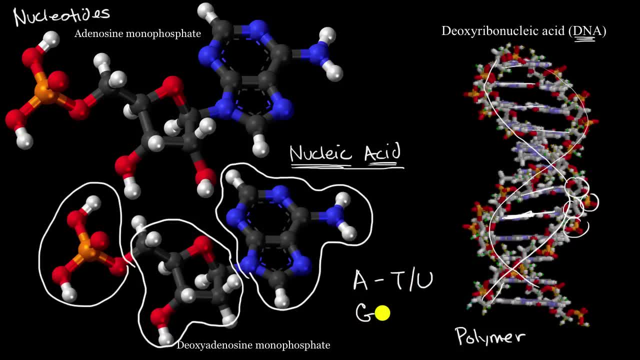 it's a nitrogenous base known as uracil, and adenine matches with cytosine. Don't worry too much about this now. We'll go into some depth in this in future videos, when we talk about DNA and how information is stored in it. 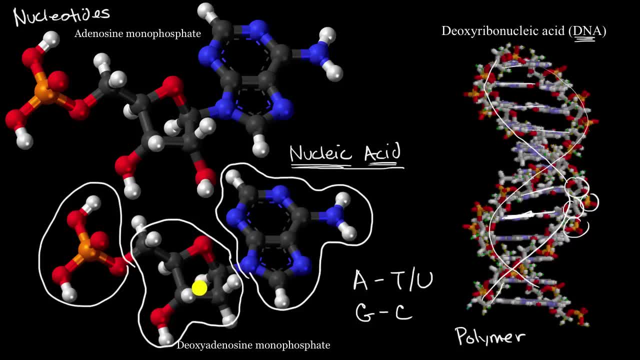 but for the sake of this video, just appreciate that the monomer for a nucleic acid like DNA is a nucleotide, so monomer, and, to be very clear, this would not be the only monomer: The analogous nucleotide in RNA. 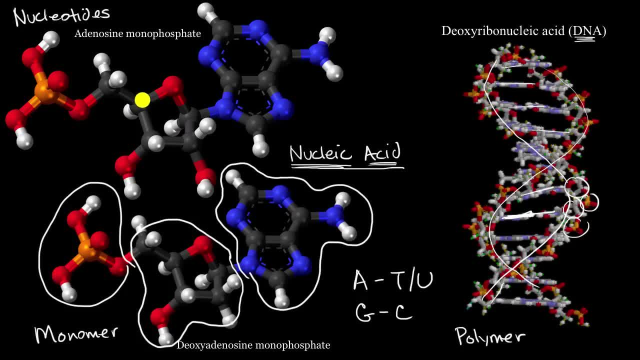 which stands for ribonucleic acid, would be adenosine monophosphate right over here. You can see the difference between the two, that we have an oxygen right over here and we don't have an oxygen right over here. That's why this is called deoxy. 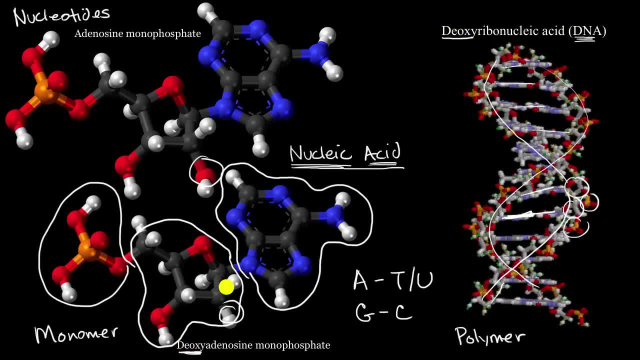 and that's why it's deoxyribonucleic acid. You're missing one of those oxygens on your five-carbon sugar. but adenine, as I mentioned, is not the only nitrogenous base. You could have a nucleotide. 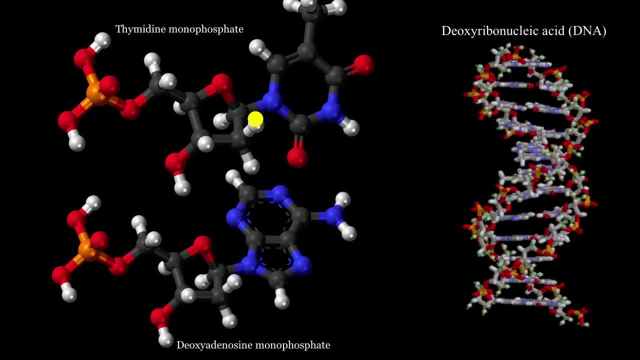 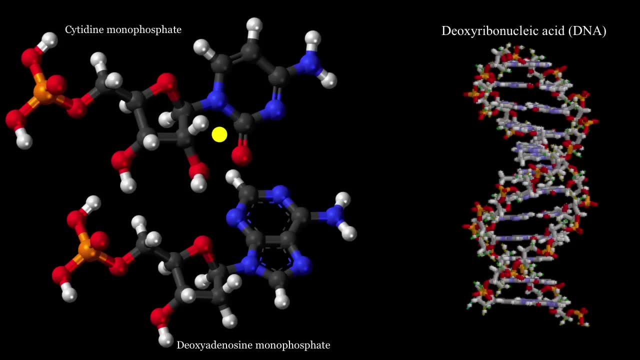 where the nitrogenous base is thymine, and so once again, this looks very similar, but notice what is going on over here. You could have a nucleotide that looks like this. Once again, you have your five-carbon sugar here. 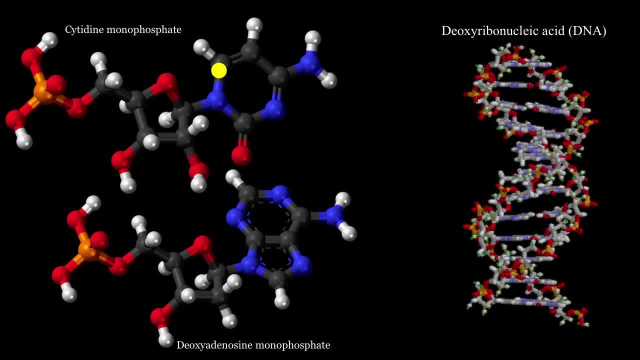 you have your phosphate group, but the nitrogenous base here keeps on changing, and it's the order of these different nucleotides that actually encodes the information in DNA. Now one question you might say is: well, look, if I have this part of the molecule. 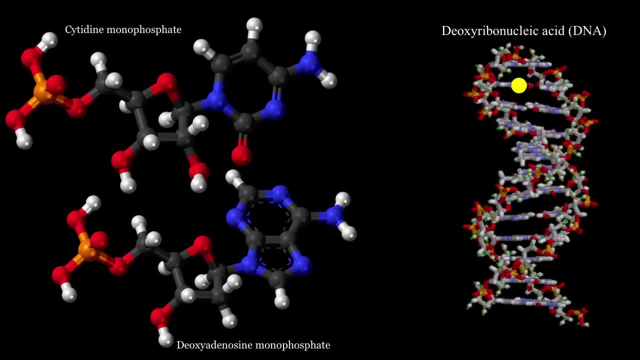 that has basic characteristics. why is it considered an acid? Well, look at how this molecule is structured. The basic parts form the rungs of this ladder, so they're not going to be as reactive because they're really tied. they're closer to the inside of the molecule. 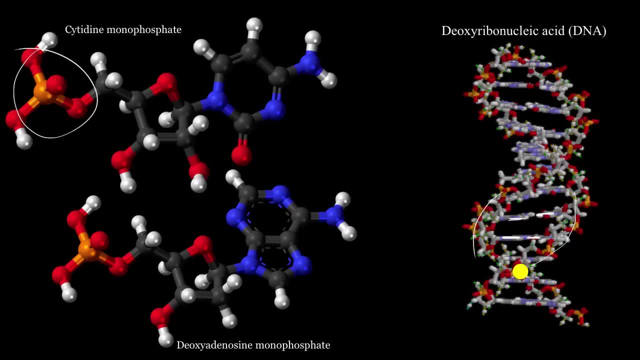 while the acidic parts, the phosphate groups, are on the outside, so they're going to be more reactive, and so the molecule as a whole is going to have an acidic characteristic. I'm going to leave you there. In future videos we're going to go into a lot more depth. 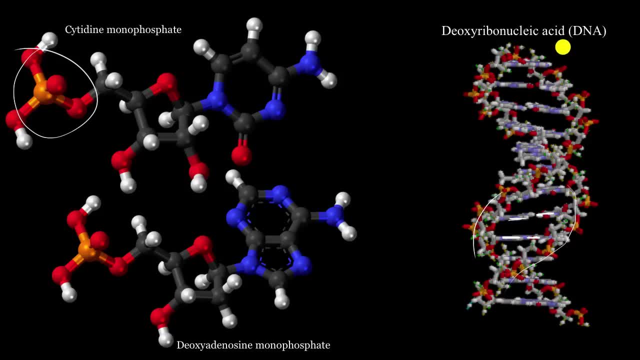 in the importance of nucleic acids, especially DNA and RNA, and to just to appreciate how amazing these molecules are. some folks theorize that the first signs of life were nothing more than self-replicating RNA molecules that eventually got enclosed in some type. 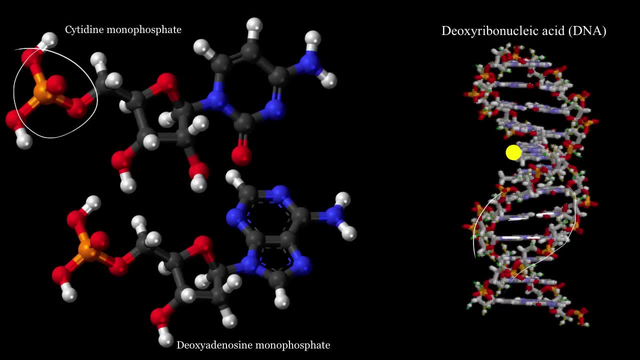 of membrane structures which eventually started forming the genetic machinery of a cell, et cetera, et cetera, et cetera. so this is why these nucleic acids are sometimes considered the most fundamental macromolecules to life.